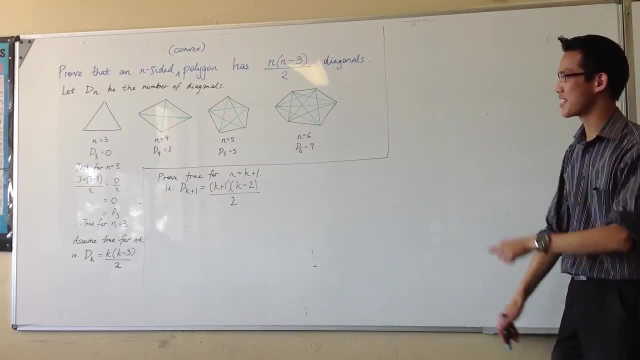 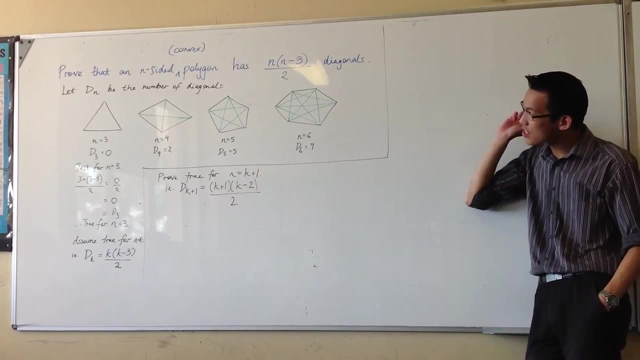 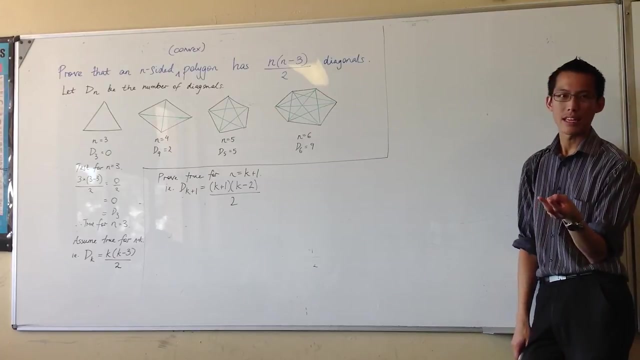 I started it as induction proof, right. The reason why is because, even though the question didn't say: do it by induction, why not right? Because induction is a method of proof and, as the question's sort of set up number one, you already know what you're trying to prove. that's a requisite for induction. Number two: you're dealing with integer values. Induction doesn't have to deal with integers, but it usually does, right. 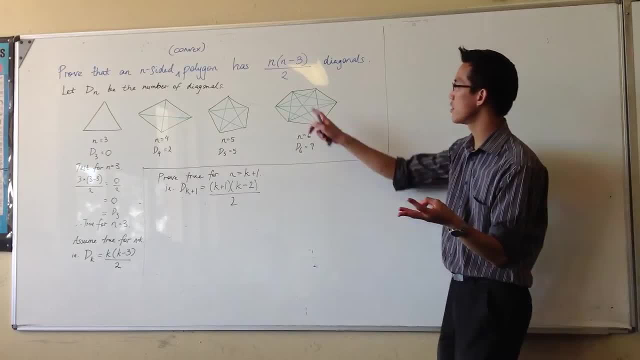 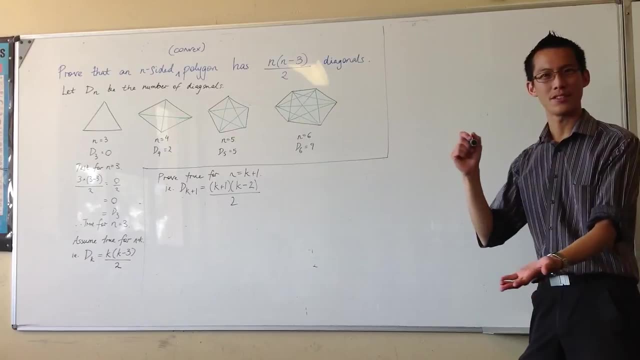 And number three, when you're, you don't just know this, you actually know all the intervening values right, So you can test things out. So that's why this question is sort of induction shaped. even though they don't say you know, prove it this way. 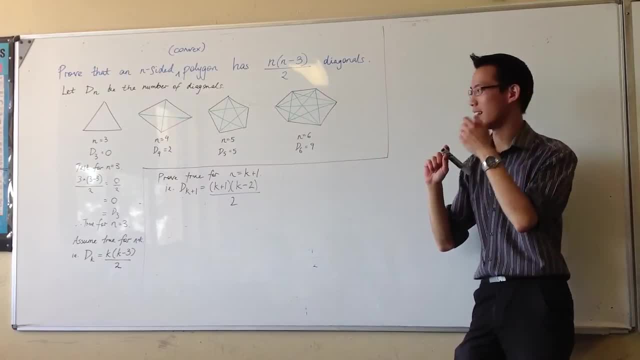 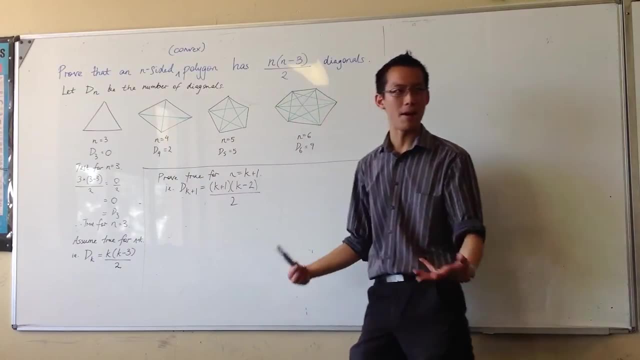 So I just thought I'd draw something out, even though that doesn't necessarily contribute to my solution, because it helps me wrap my brain around what's happening. And then you can see I've just sort of started out my first three steps. right, So test it. 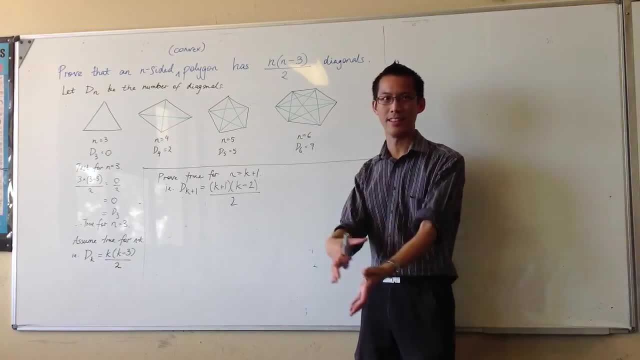 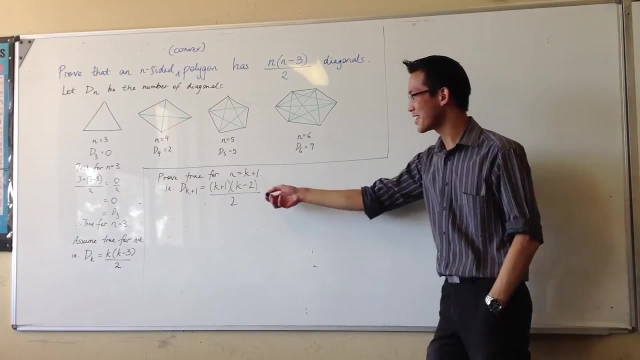 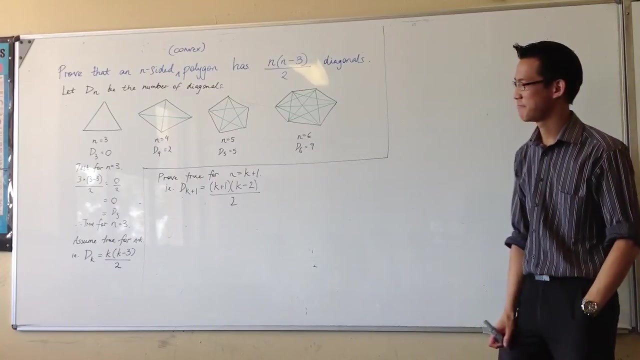 First of all, the value I just put is three, because if you have anything less, you're going to have to do it again. If you have anything less, you don't really have a polygon, right. Then I assume- now I have to prove this is the fun part right Now, when you look at this- how could you possibly work in your assumption into here? That's the real, that's the question, right? Does anyone have any ideas? How would you go about doing it? 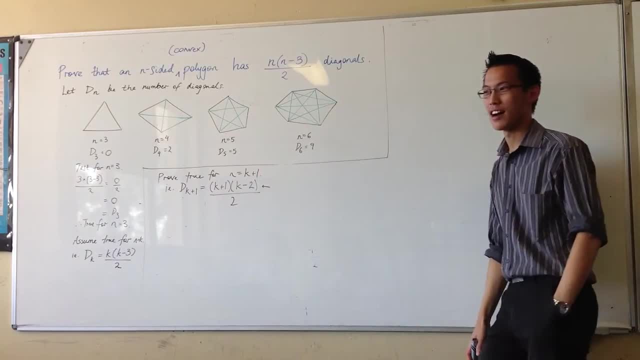 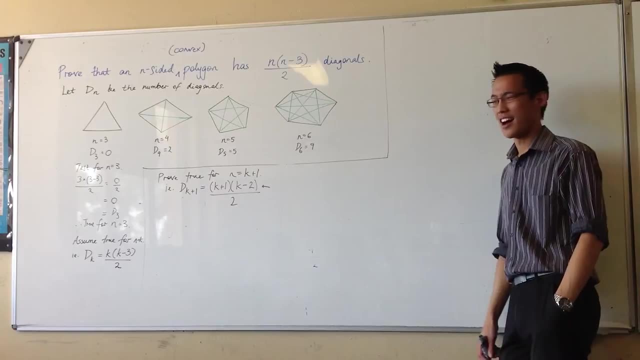 This thing. here I could expand. It would end up with something that I would argue is no more complicated or no more simple than what I'm going to get in a second, So I'm going to leave it factorized for now. I think it really depends on this thing. 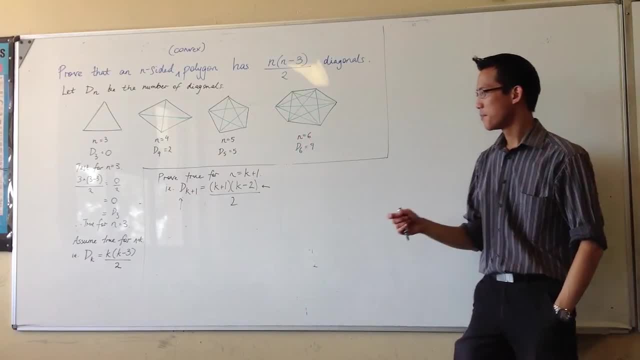 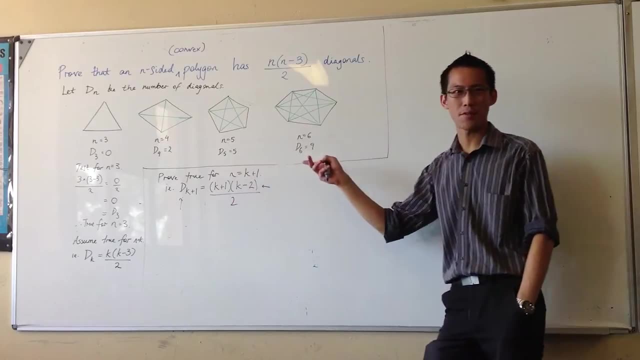 It has to come from there somehow. okay, Because if I'm going to bring this in, right, I don't have it on the right-hand side. Even if I did have it on the right-hand side, what would it achieve for me to bring it back in? okay? 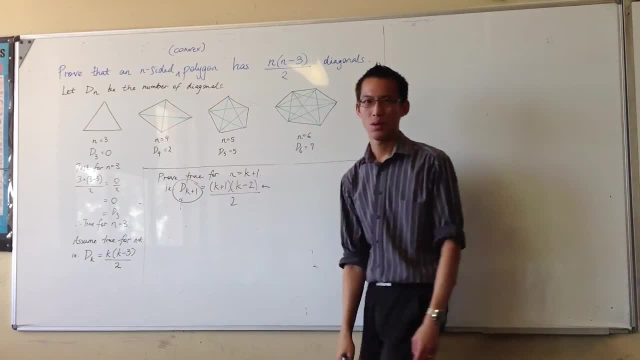 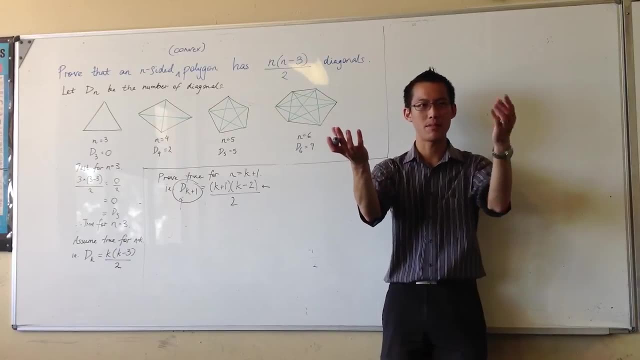 So I think the key is to really understand what happens when you go from- I'm just calling capital D, the number of diagonals, I've got right- What happens when you go from one k to the next, one k plus one? 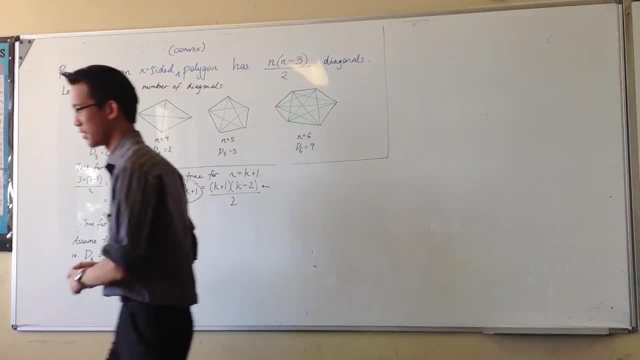 Well, that's why it's actually useful to have this diagram, okay, or this set of diagrams, Because you can see a pattern, can't you? You can see a pattern As you go from one to the next: what's changing in the number of diagonals? 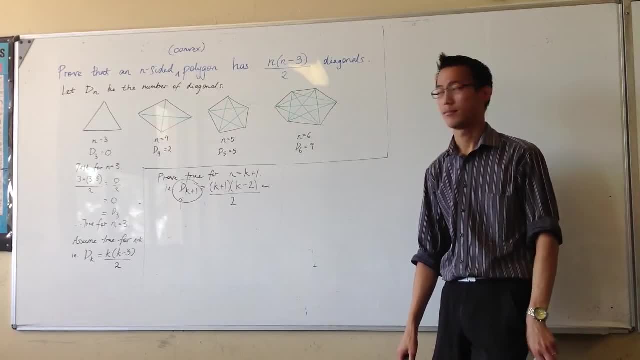 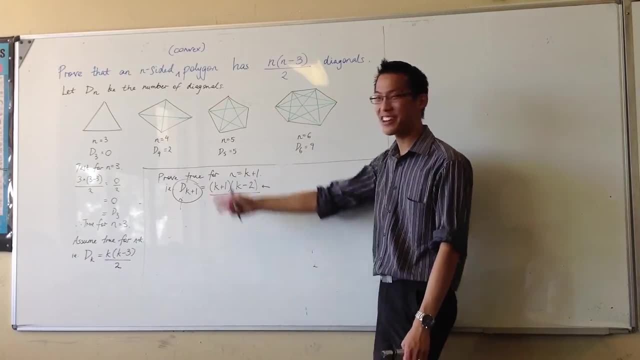 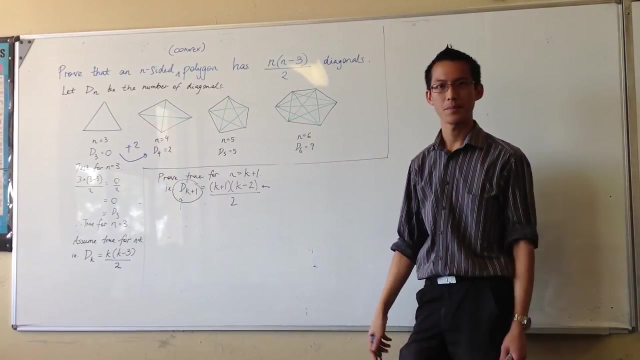 Well, it's getting more, but for how much? As you add in one vertex, as you add in a corner right, you go from zero to two right Plus two diagonals. okay, As you move over from four to five, you add how many diagonals? 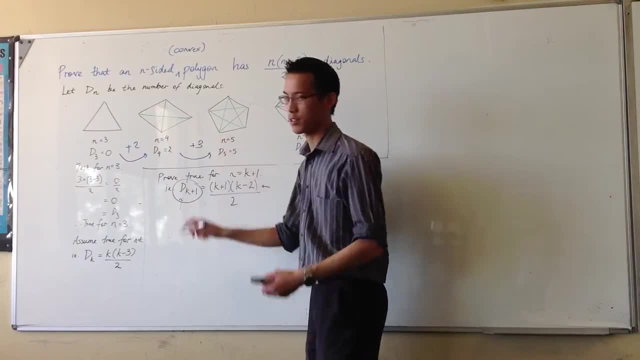 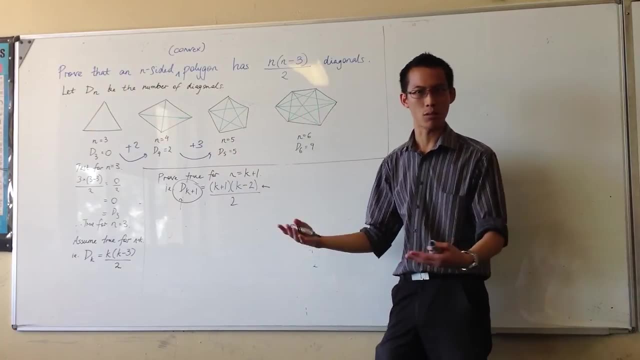 Three, right Now, by the way, because the pattern is starting to come out. why is it that this number that we add on is so methodical, right? Well, two reasons. Number one- and you can sort of see it because I've got enough diagrams here, right. 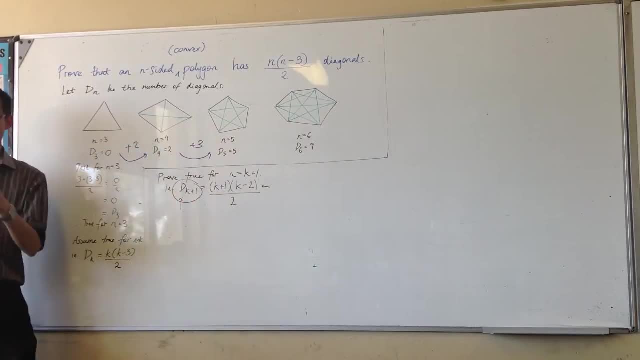 Number one, you've got more vertices to draw out diagonals to other places, right? Because if you think about it this way, Number one, you've got more vertices to draw out diagonals to other places, right? Because, if you think about it this way, 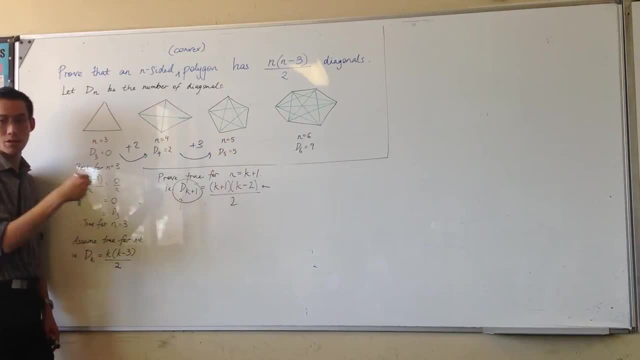 I started here and I drew one and then I drew another one. so I drew it twice right From two starting points and then I was finished. There were no more diagonals I could draw, But when you go for this one, 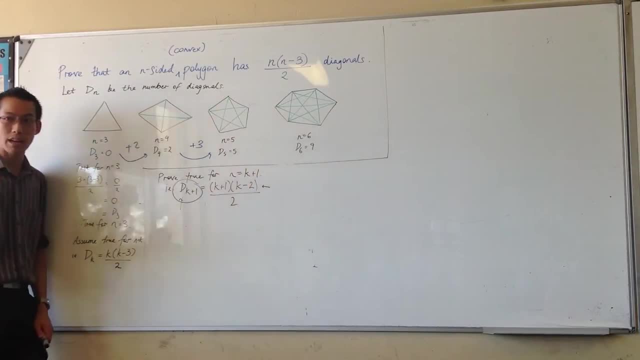 you're adding in an extra point that can go to more places, right, So you've got more starting points. But secondly, can you see the other thing that's growing As you go from here to here to here? each corner, right? 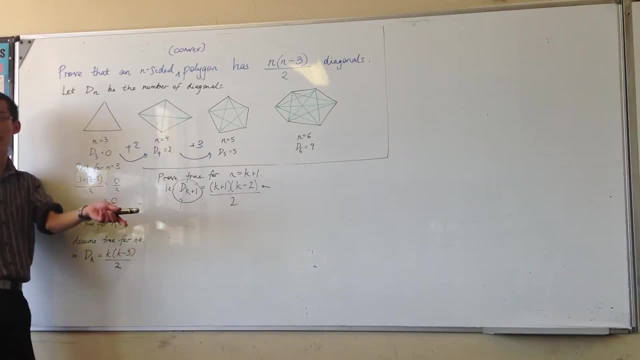 not only are there more corners, but each corner sends out more diagonals, right? See, here I've got one diagonal per corner, There's just one coming out. Then you've got two. Every corner has two diagonals. And then here you've got three, right. 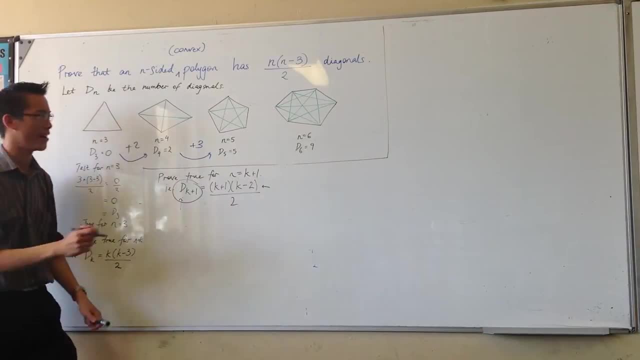 So that's why it's growing in this very sensible way. okay, So from here to here plus four. Now what kind of series is this? Now, this series in here? that's arithmetic right. Common difference of one. 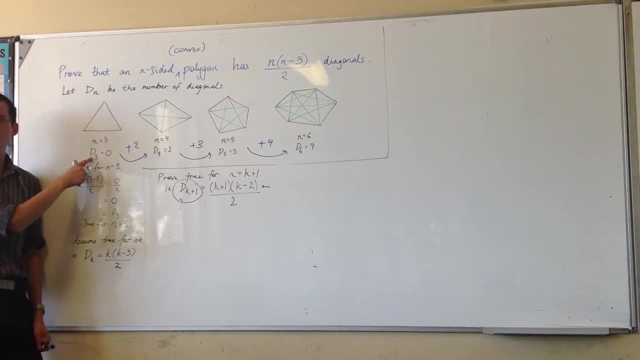 But the actual series I'm interested in D is not arithmetic, is it Like it's just? It's just a series. It's not arithmetic, It's not geometric, It's just that okay. So if I want to try and break apart that series, how would I do it? 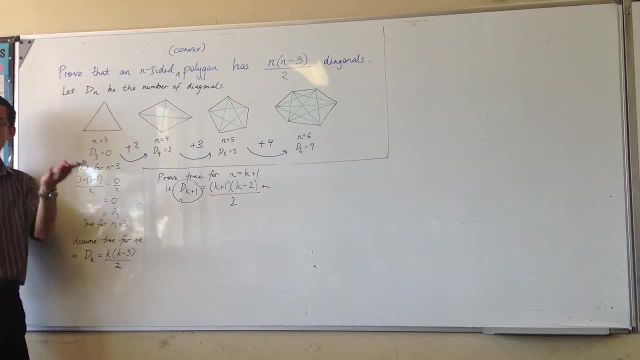 I can't use my normal rules, or formerly for APs or for GPs. So what do I do? Hmm, Well, I'm going to say: here's my left-hand side. okay, That the k plus one-third term. 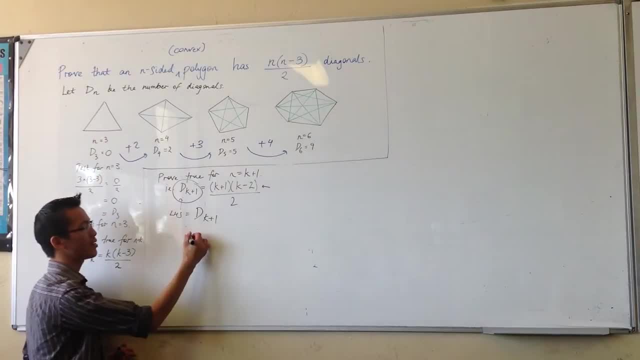 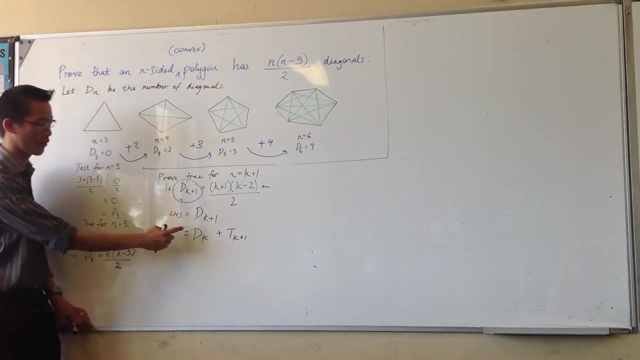 whatever it is, whatever rules it follows- right, It's going to be the previous, well, the previous k terms. right, That one Plus whatever the next one is Normally that Okay. Does that make sense? So, for instance, if I was looking for the 100th term, 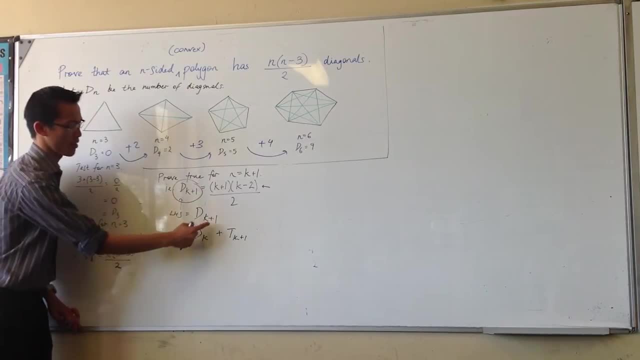 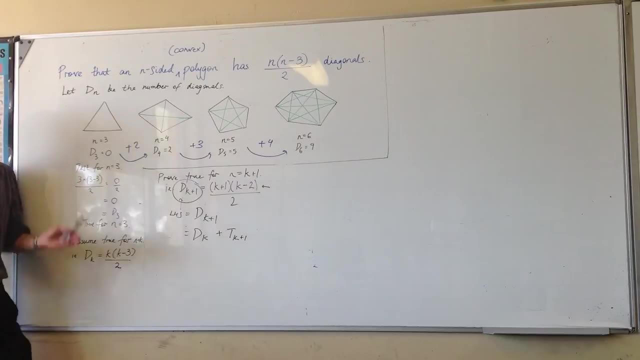 it would be the first 99 terms, sorry, the first 100 terms. It would be the first 99 plus the 100, right? So that's my k and that's my k plus one right Now. this is useful because I'm trying to work in my assumption, right? 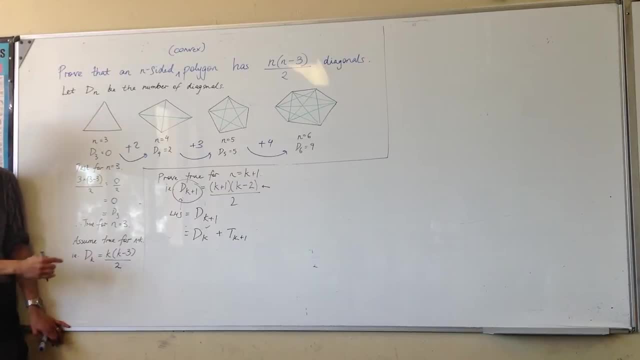 So that's good. okay, I've got my D d k there, But in solving one problem bringing it in, I've introduced another one. What is this thing? What is k plus one? How do I go about finding it? 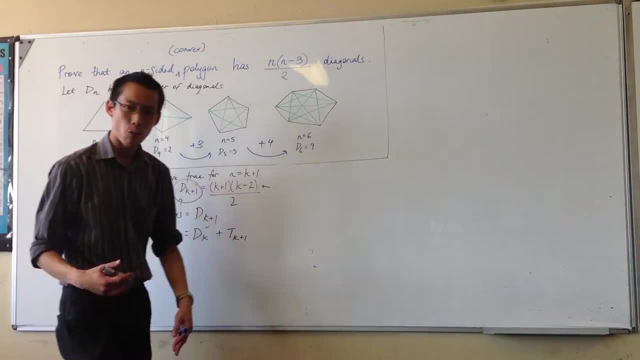 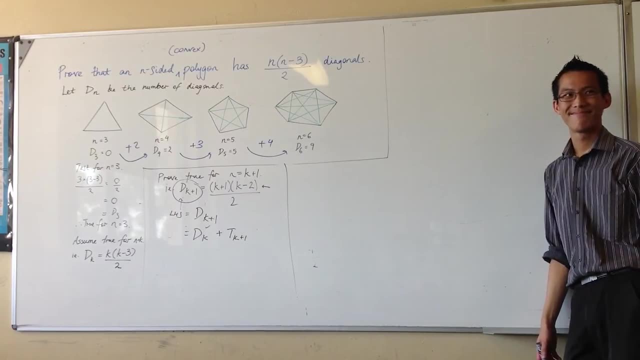 Remember, it's not an AP or a GP, right? So we can't use our ready-made rules for those. What else can I do? Observe the pattern, Exactly right, right, So I want to watch what's happening here, okay. 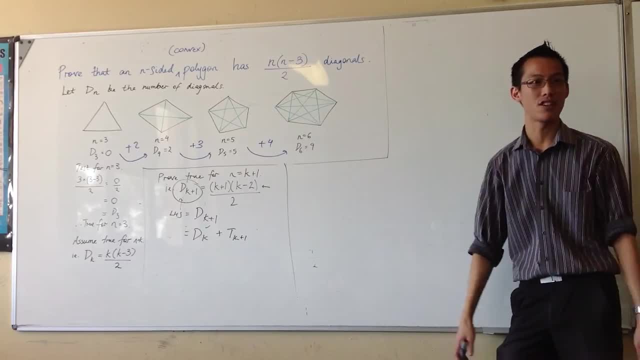 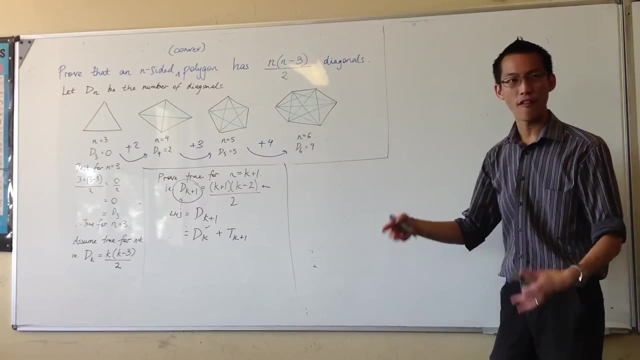 And you can make some educated guesses. I'm going to go straight for the algebra, okay, Because not only can I observe the pattern, I already have an algebraic expression for the pattern. okay. So I'm going to say: if I want to work out t of k plus one, 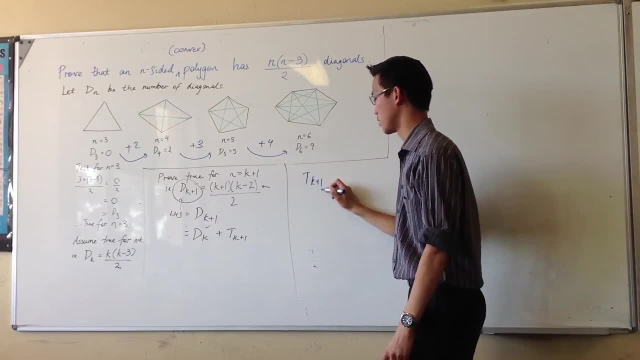 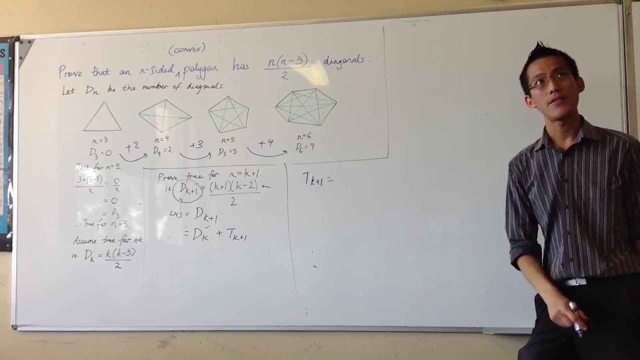 I'll put this off on the side. okay, t of k plus one. okay, If I want to work out, say, the 100th term, a way of thinking about that is well, if you take the first 100 terms, okay. 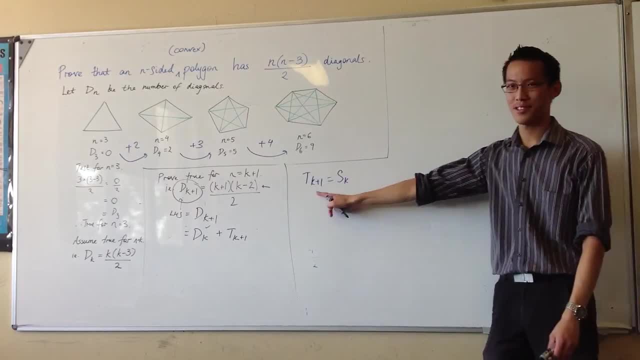 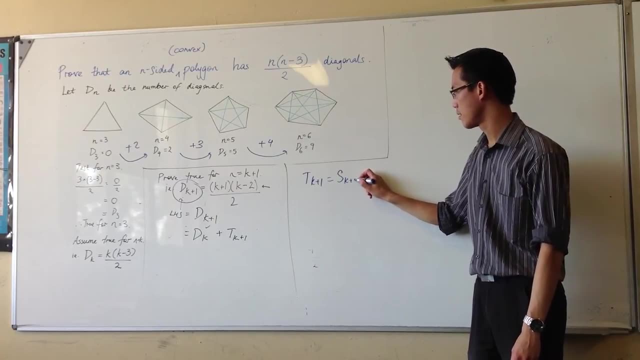 and then you subtract all the ones except for the one you're interested in, right t of k plus one. So I should have done this. I think That's what I wanted. okay, Can you see what I'm doing here? okay? 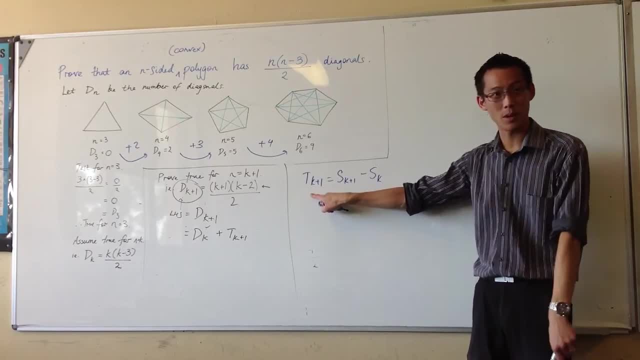 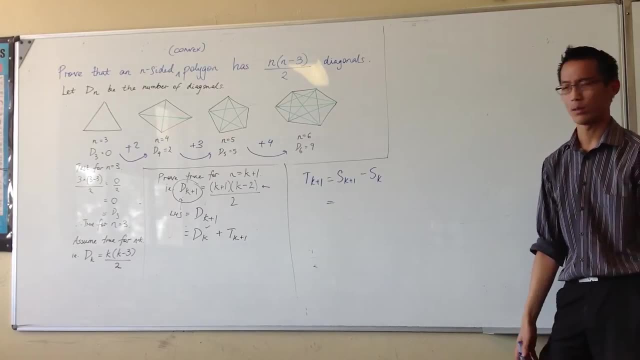 I'm taking the sum of every term up until this one, and then I'm taking away all the previous ones, all the ones I don't want, right? So what does this land on? What does it look like? Well, I know what all of these pieces are. 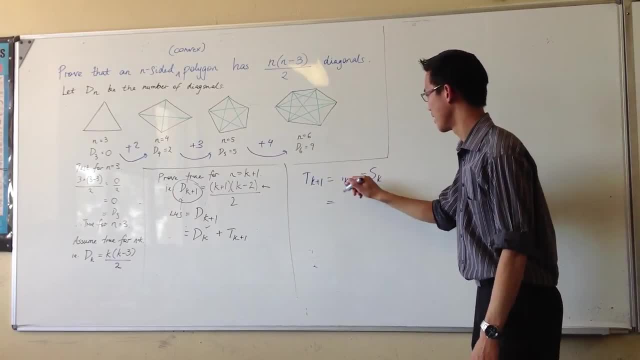 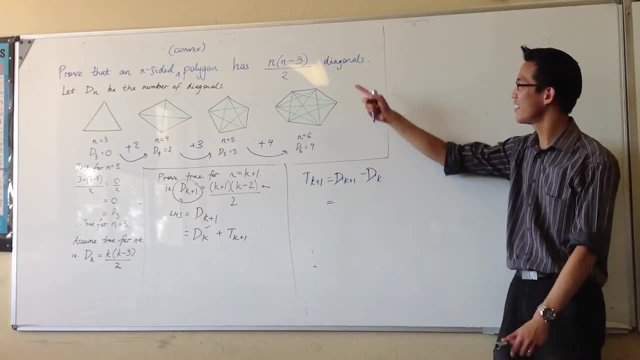 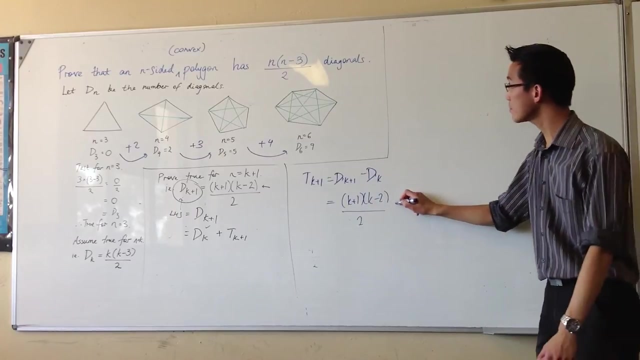 because I defined them that way, right, Sorry, this is a d. I keep on thinking of sum. Okay, does that make a little more sense? okay, So d of k plus one is going to be k plus one. k minus two on two. yep. 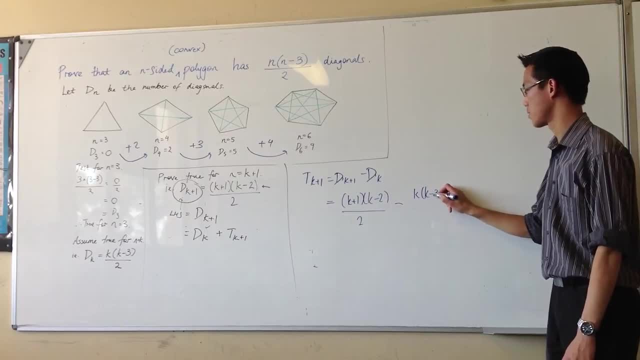 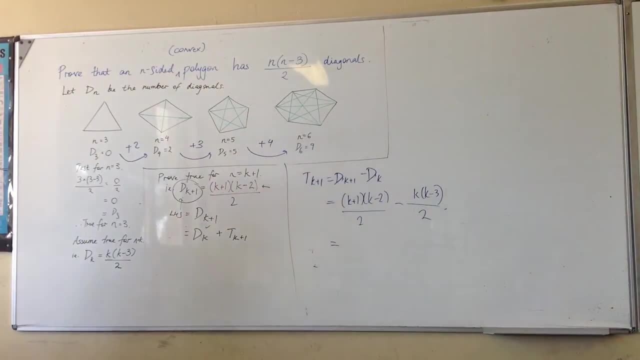 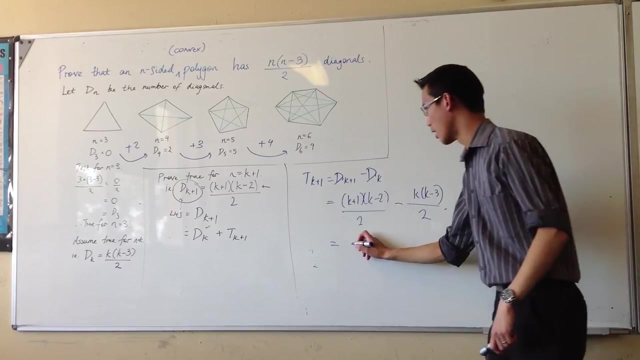 And I know what this is already. That's k k minus three. Okay, off you go. What does it work out to You? tell me, 2k minus two, 2k minus two, Because I've got here what I've got. 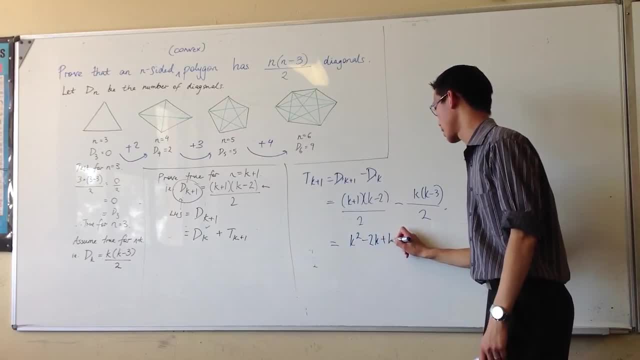 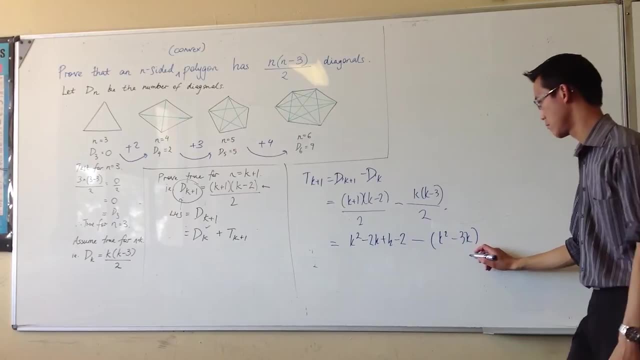 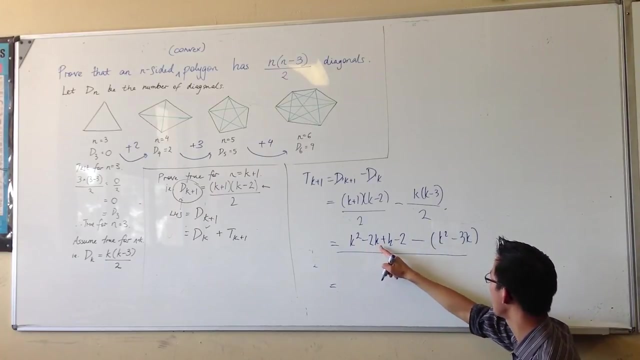 k squared minus 2k, plus k minus two, minus k squared minus 3k. Yeah, All one two. That's just one fraction. Yes, Okay, so I've got k squared minus k, so this k squared will cancel with this k squared. 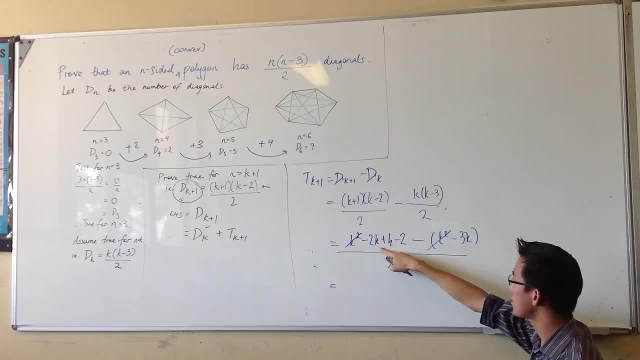 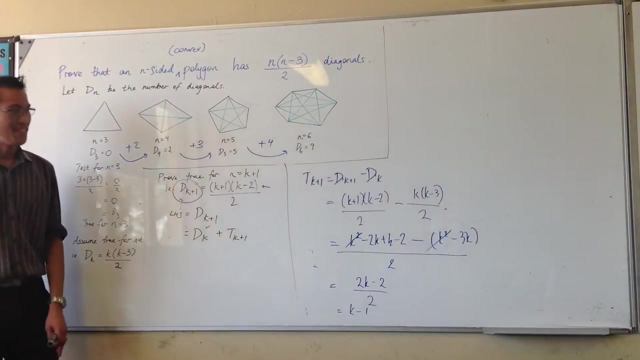 Yeah, I've got minus k here plus 3k, So 2k minus two, Yeah, And that's actually all over two. So, if I should, So k minus one, Okay, Now does that make sense? Of course it makes sense. 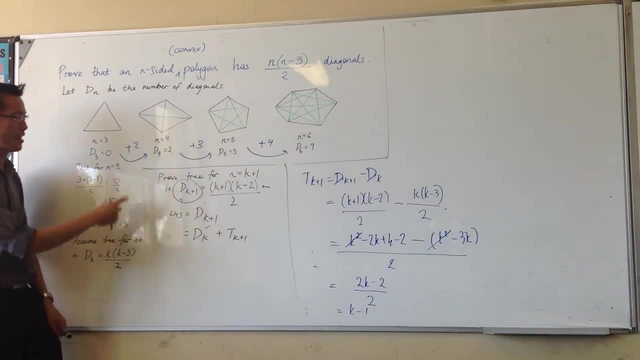 because k minus one is exactly what we're adding as we're going from term to term, right Two and then three and then four. Okay, You see how it's going in the same way. All right, now I can actually put this into place. 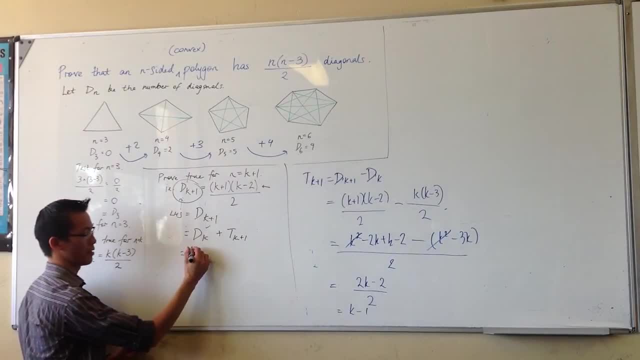 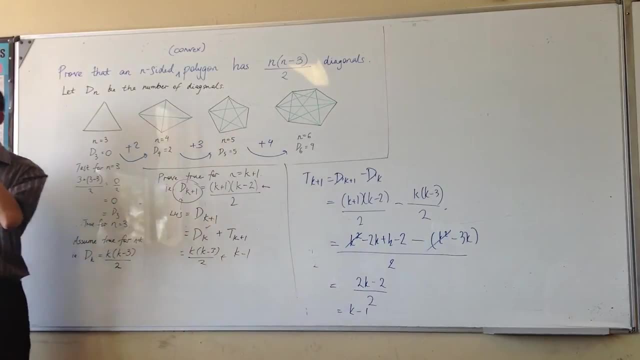 So here, what have I got? k minus three, Right, Does it fit? Where do I want to go? Where do I want to go? This is going to be two on two. Yes, So I've got k squared minus three. 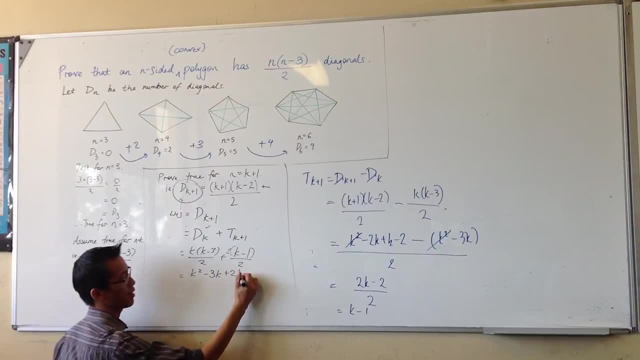 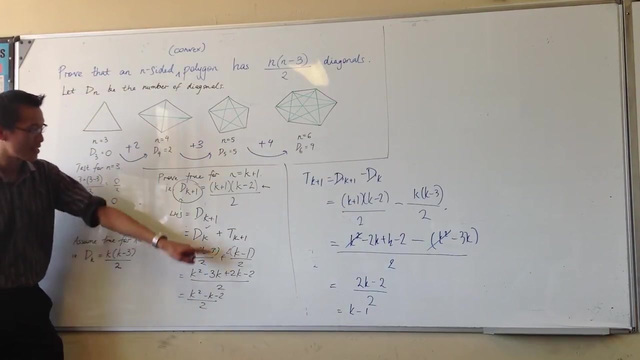 k squared minus three k plus 2k minus two. All over two k squared minus k minus two. Does it check out, Ta-da? I actually I should have left myself a line, but that's going to end up here. 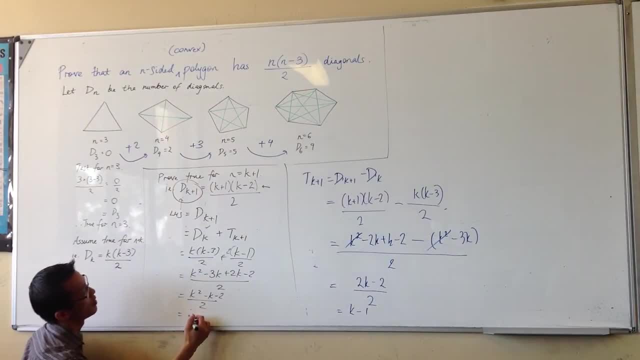 the factorized bit that I was after. Right, That's equal to- I can just fit it, Ta-da, What I was after. Okay, Now Yeah, Are you allowed to make that assumption of the k plus one, because that's what your proof is? 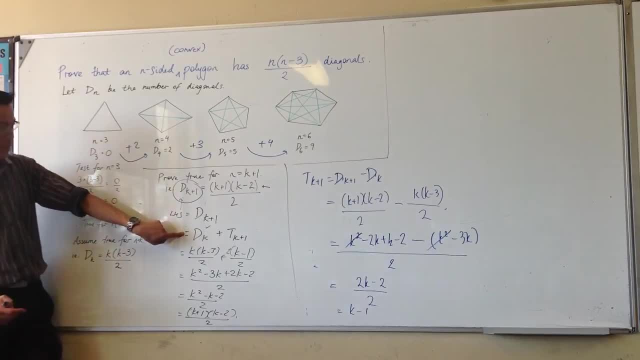 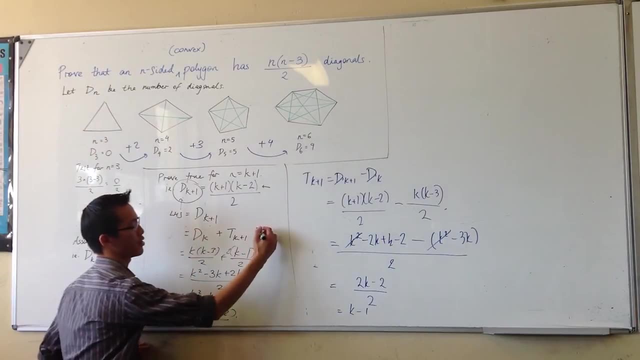 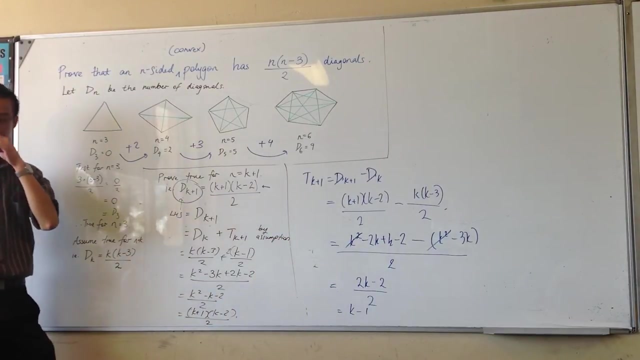 Yeah, This part here. Okay, So two things. I am assuming what d of k is. That's my inductive step, right? So I really should have said my assumption here, Because if you substitute t k plus one equals d k plus one minus d k. 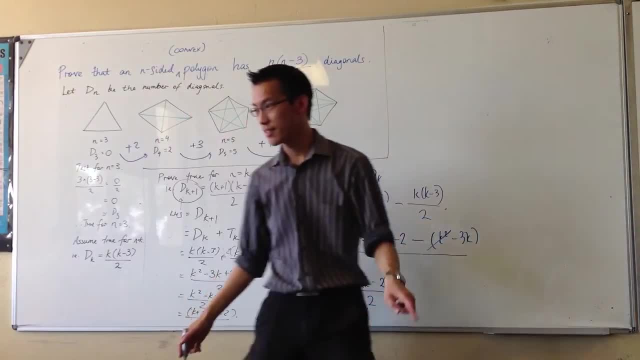 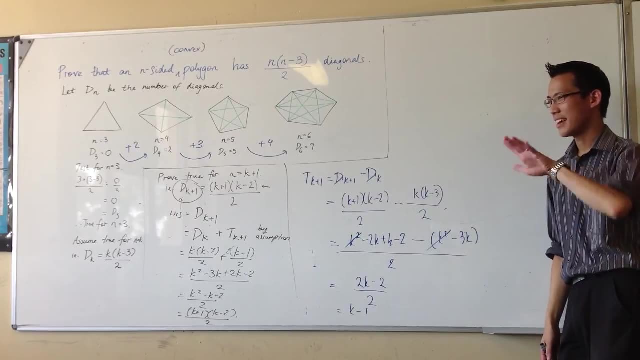 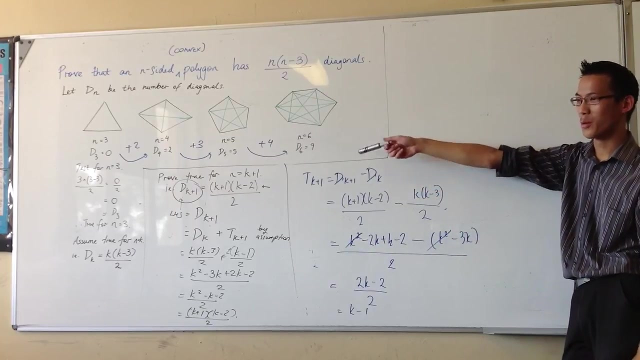 doesn't that just cancel, You mean from here? No, if you substitute that top layer into that, This one, Yeah, Okay, Yes, but no, Because I'm not assuming that this is true. Right, I'm actually working it out based on what kind of 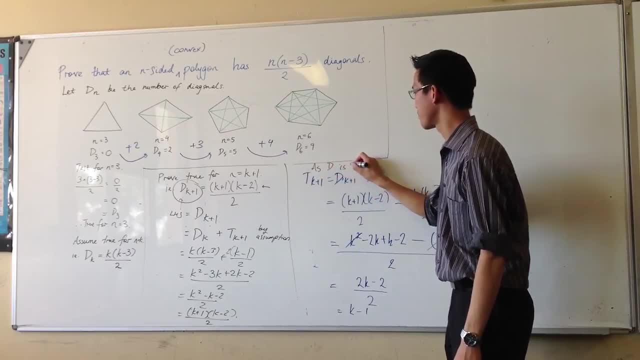 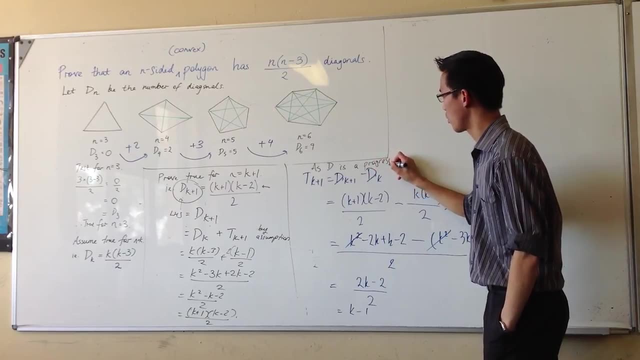 So I should have said, as d is a, What's the word I'm looking for? Is it a progression? That's all I want? Okay, Right, Because that's the definition of something which is progressing from term to term, Right. 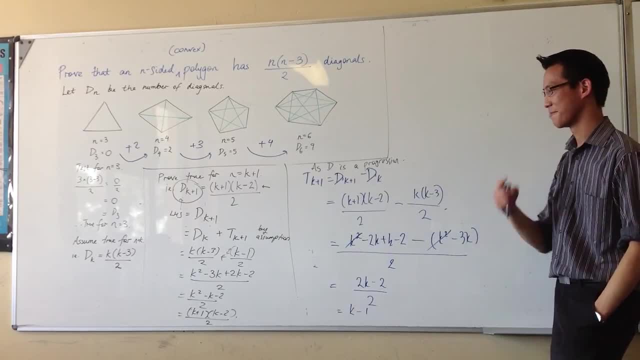 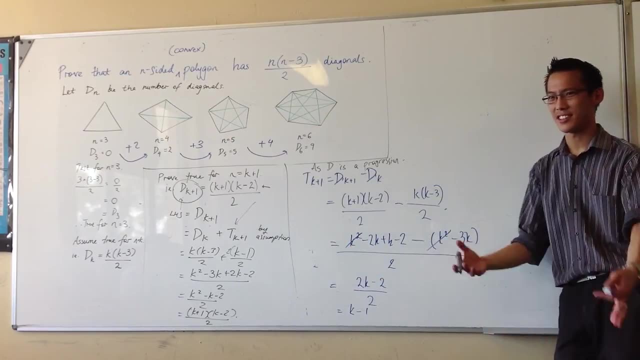 So that's why it's not as circular as it looks. Okay, I think the hard part was here, That one, The actual step we're talking about. Okay, Because it's not intuitive that you'd go in that direction. And how else do you break apart this guy? 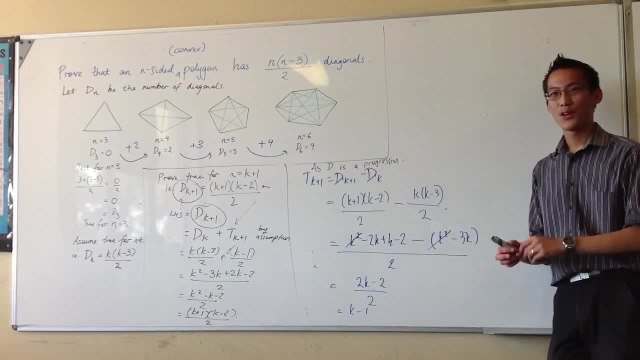 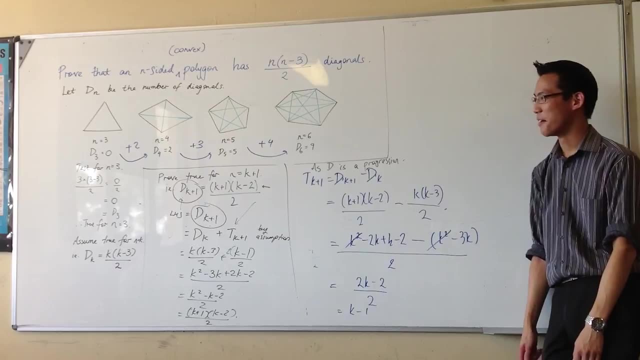 That's the hard part. Okay, Now you guys got lucky. There were no geometry induction questions For now. When your trial rolls around, they'll make another appearance, Because in your HSC they'll make another appearance, Actually, if you go. 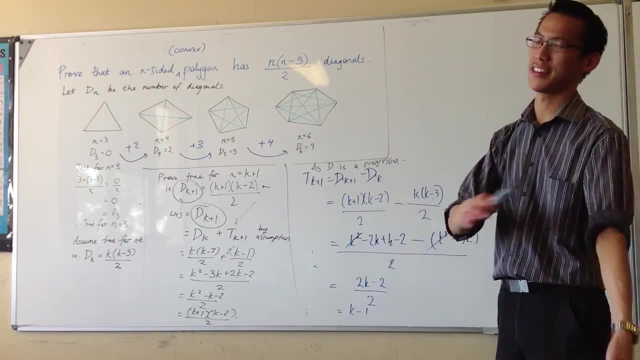 when we get to the time when we get to look at real HSC exams, you'll see lots of geometry induction questions in there, Because geometry induction questions are hard, So that's why they make you do it, Okay. So anyway, Thank you.